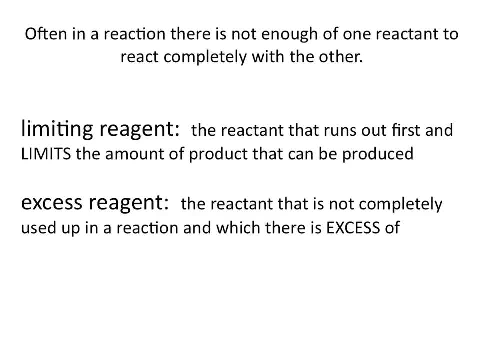 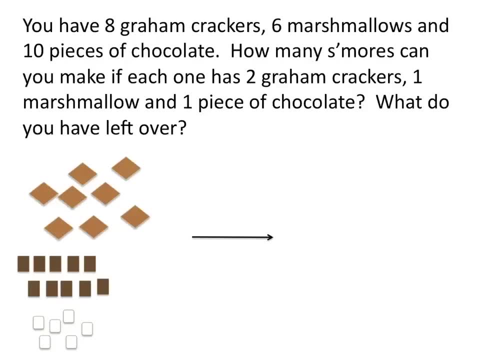 that can be produced. The excess reagent is the reactant that is not completely used up in a reaction and which there is excess of. Let's look at a non-chemistry example first. You have eight graham crackers, six marshmallows and ten pieces of chocolate. How many s'mores? 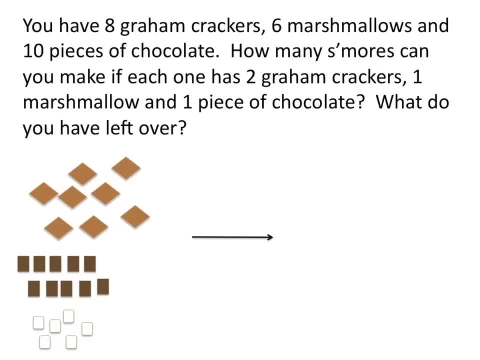 can you make? if each one has two graham crackers, one marshmallow and one piece of chocolate? What do you have left over? So you'll see that we can make four s'mores and we have six pieces of chocolate left over and two marshmallows left over. 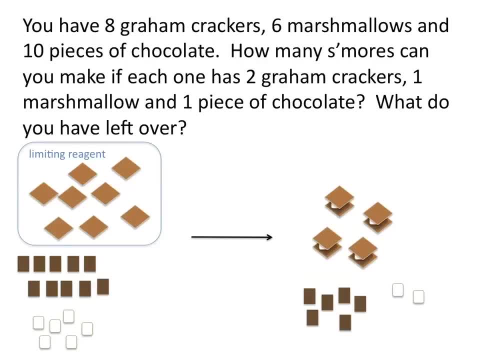 What makes the graham crackers the limiting reagent, Or the reactant that we ran out of first and which limits the amount of s'mores that can be made. The chocolate and the marshmallows are both excess reagents because we have extra of each of those. Now let's look at a more. 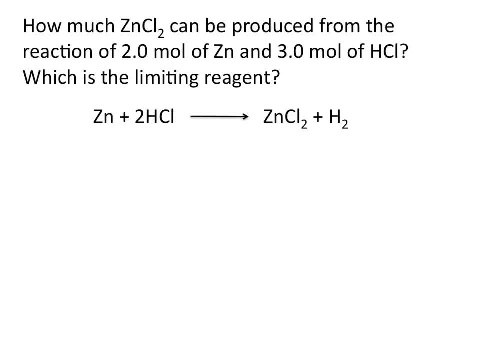 chemistry. specific example: How much zinc chloride can be produced from the reaction of two moles of zinc and three moles of hydrochloric acid, Which is the limiting reagent? For your first step, you're going to check for a correctly balanced equation And in 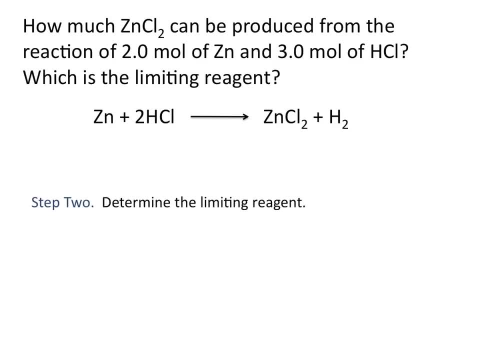 this example, our reaction is already balanced. The second step is to determine the limiting reagent, And we can do this one of two ways. The first way is to determine how much product can be made from each of the given reagents. First, let's start with our two moles of zinc. 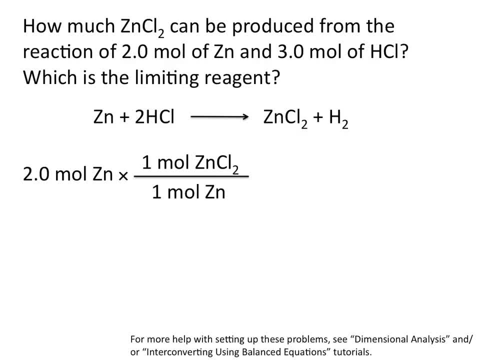 In order to convert moles of zinc to moles of zinc chloride, we need to use the coefficient in our correctly balanced chemical equation. This tells us that one mole of zinc is required for every one mole of zinc chloride that is produced. Now remember: you can only convert. 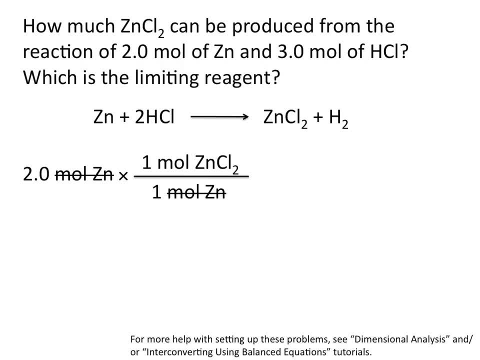 from moles of one reactant or product to moles of another reactant or product. So if you were given amounts in grams, your first step would be to convert those amounts in grams to moles, And then you can use the coefficients in your balanced chemical equation. This tells: 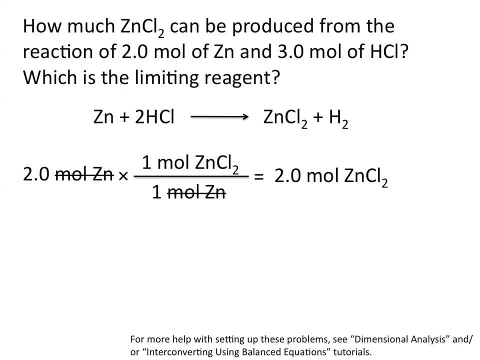 us that two moles of zinc And excess hydrochloric acid can make two moles of zinc chloride. Now let's look at how much zinc chloride can be made from the three moles of hydrochloric acid that we start with. Again, we'll use the coefficients in our balanced chemical equation, which tell: 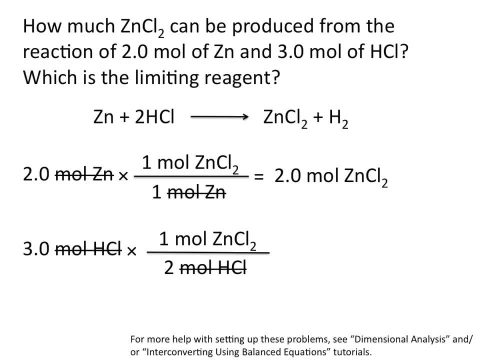 us that for every one mole of zinc chloride produced, we need two moles of hydrochloric acid. This tells us that with three moles of hydrochloric acid and excess zinc, one point five moles of zinc chloride could be produced. Now what you'll notice from these: 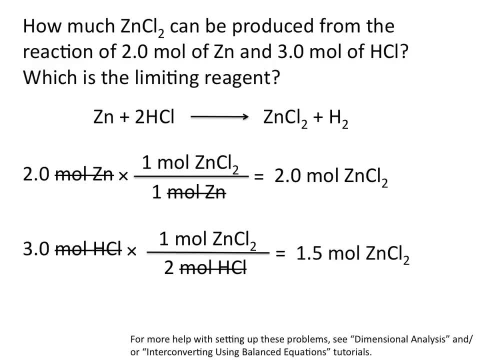 calculations is that three moles of hydrochloric acid can at most produce one point five moles of zinc chloride, So it doesn't matter that we have extra zinc. And so even though our two moles of zinc could theoretically make two moles of zinc chloride in this reaction, 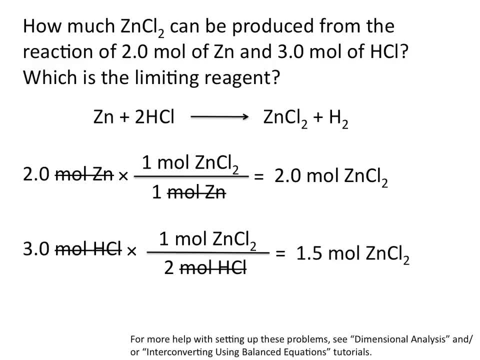 the hydrochloric acid will run out first, after the production of one point five moles of zinc chloride, And this is our theoretical yield. This makes HCl the limiting reagent, And so, in this equation, the three moles of HCl. 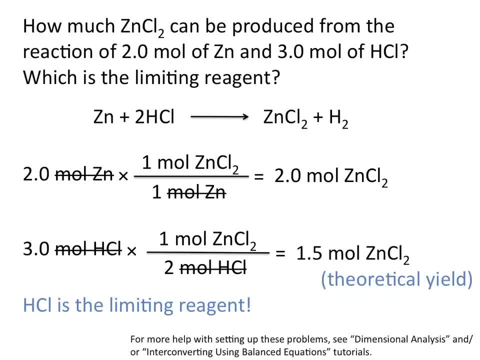 would react with zinc in order to form one point five moles of zinc chloride, And this would mean that you would have excess zinc left over, because there was no more hydrochloric acid left for the zinc to react with. And even though this problem doesn't ask for our 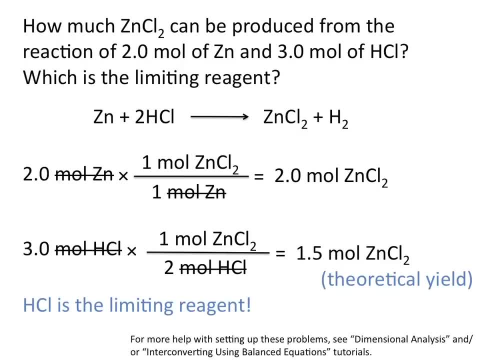 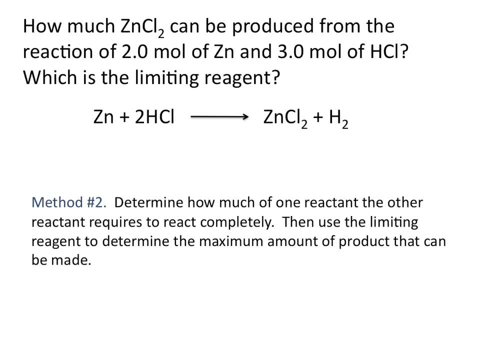 excess reagent. this means that zinc is the excess reagent. Another method that you can use to determine the amount of hydrochloric acid that you want to produce is called the limiting reagent. The limiting reagent is to determine how much of one reactant- the 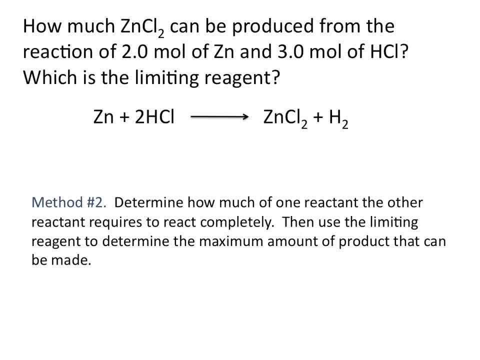 other reactant requires to react completely, Then you can use the limiting reagent to determine the maximum amount of product that can be made. So in method one we determined how much product could be made individually from each of the reactants, if we assume that they. 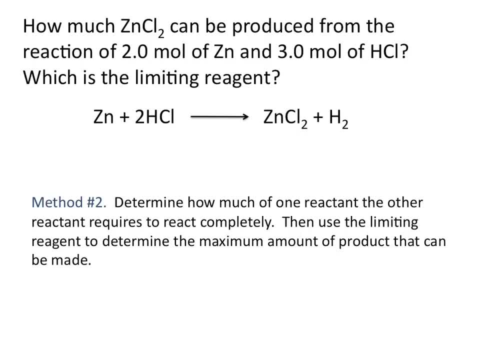 react with excess of the other reagent And then from the amount of products that can be produced, we could determine our limiting reagent. In this method, we'll determine our limiting reagent first and then use the limiting reagent to calculate the theoretical yield. You can use whichever method makes more sense to you. 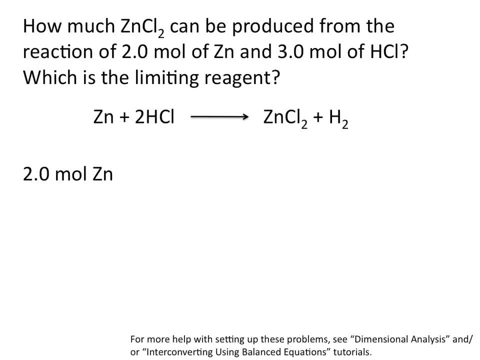 And in either case you end up doing two calculations. You can start with either the two moles of zinc or the three moles of hydrochloric acid, but I'm choosing to start with two moles of zinc. I then use my balanced chemical equation to calculate how much HCl would be required.